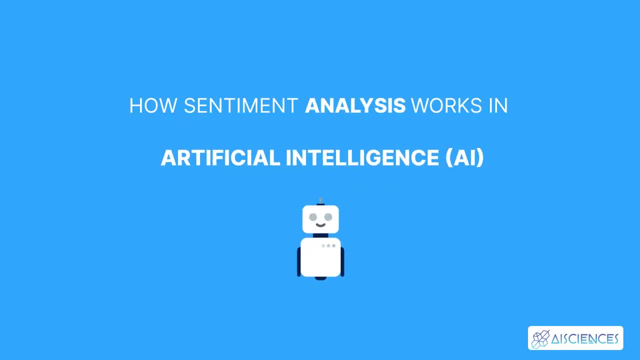 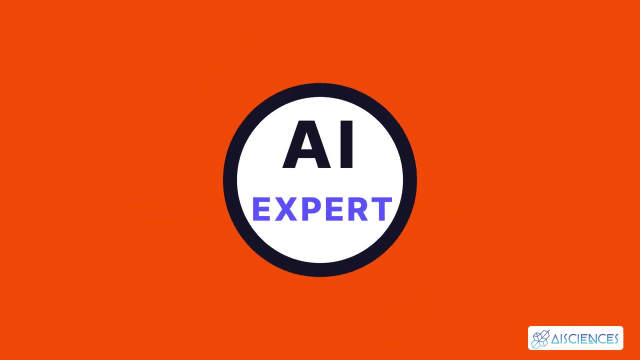 How sentiment analysis works in artificial intelligence AI. Hi everybody, If you're looking to become a full-time data scientist and artificial intelligence AI expert from scratch, then you are at the right place. Today, I'll explain how sentiment analysis works in AI. 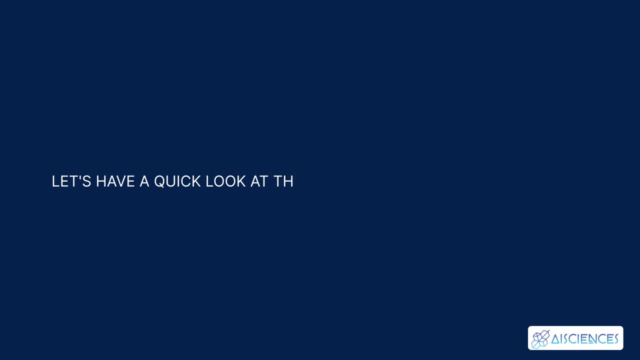 Let's have a quick look at the definition of sentiment analysis. Sentiment analysis is the process that automatically detects emotions and opinions by classifying a given text as positive, negative or neutral. But how does it work? Basically, it combines the power of two subfields. 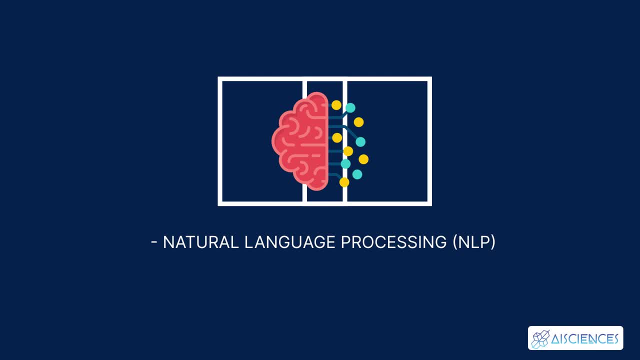 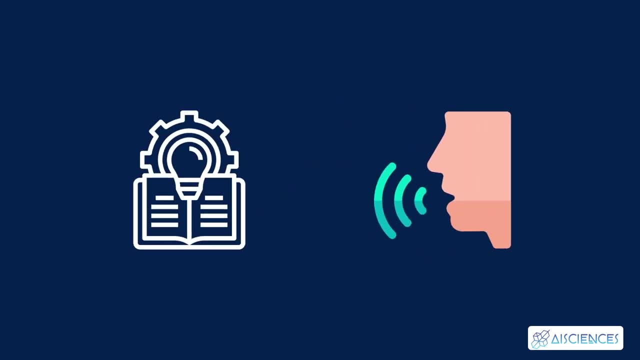 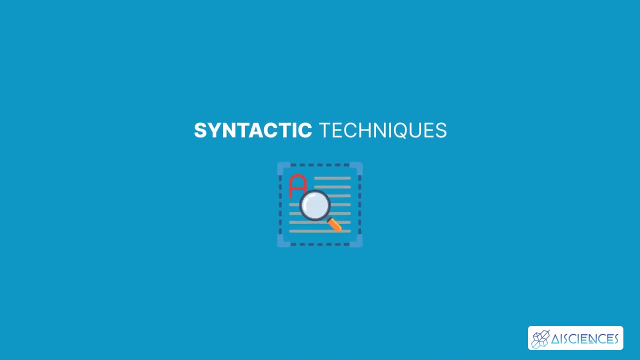 of AI, Natural language processing- NLP- And machine learning. Natural language processing- NLP transforms human language into something that machines can understand. It applies syntactic techniques to understand the structure of a text and semantic techniques to identify meaning. Some of these techniques are tokenization, limitization and part of speech tagging. 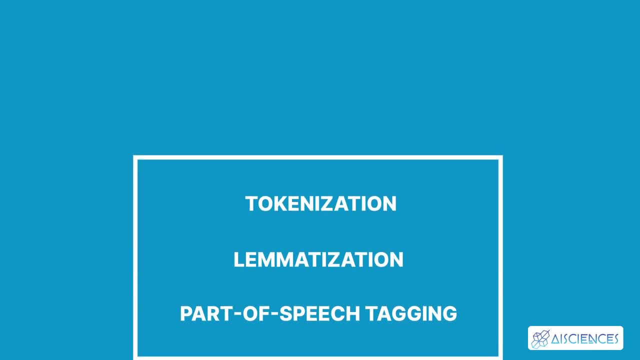 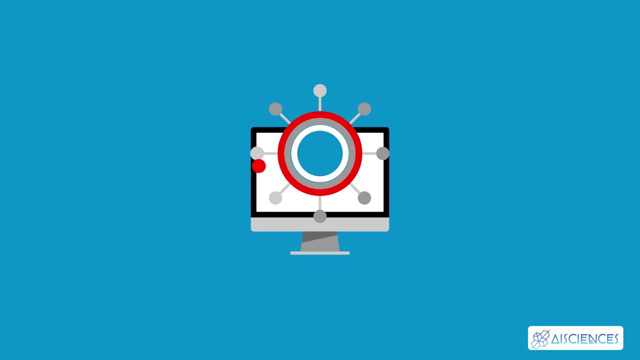 Once the text is processed with NLP techniques, it's ready for classification with machine learning algorithms. Machine learning allows machines to recognize patterns in data and make predictions Instead of relying on explicit instructions. machine learning algorithms learn from similar examples, training data To build a model that classifies text by sentiment. 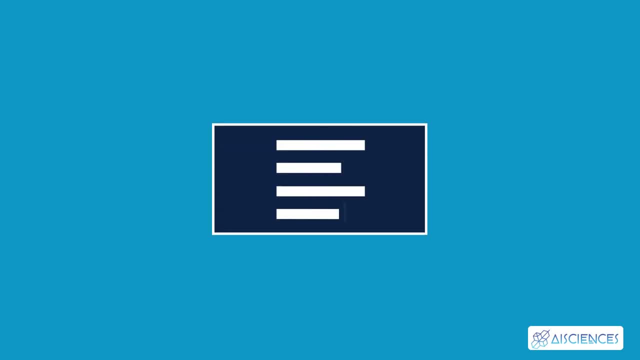 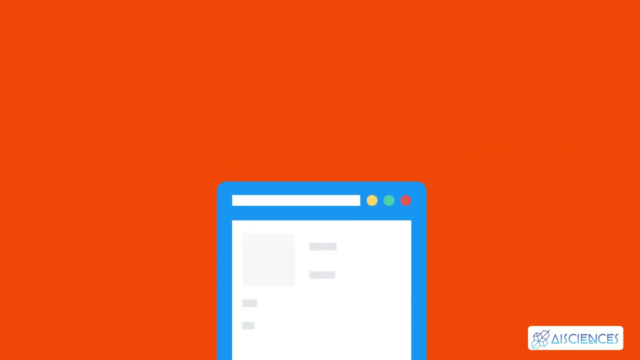 you need to train it with examples of emotions in text. These examples requires to be labeled with the corresponding category. To improve the accuracy of your model, you'll need a representative amount of samples for each tag. Looking curious about why sentiment analysis is needed In today's environment where we're suffering from data overload. 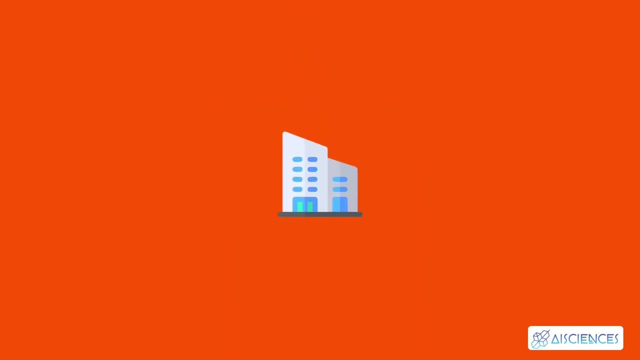 although this does not mean better or deeper insights. companies might have mountains of customer feedback collected, Yet for mere humans it's still impossible to analyze it manually without any sort of error or bias. Imagine this scenario: You're a manager of a small delivery business and you receive about 20 responses to your email surveys every month. You could read these yourself and perform your own analysis by hand. Now imagine receiving 30,000 responses per month. That's more than a thousand responses each day. Needless to say, this is impossible as a part of a business owner's day job. 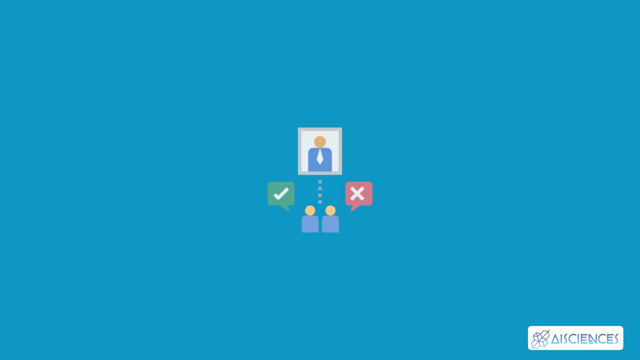 Then there's the question of bias. Everyone knows those days where things go wrong and you're in a foul mood even before reaching the office. The risk of you interpreting messages and any form of communication more negatively is rife. Sentiment analysis is useful for quickly gaining insights using large volumes of text data. 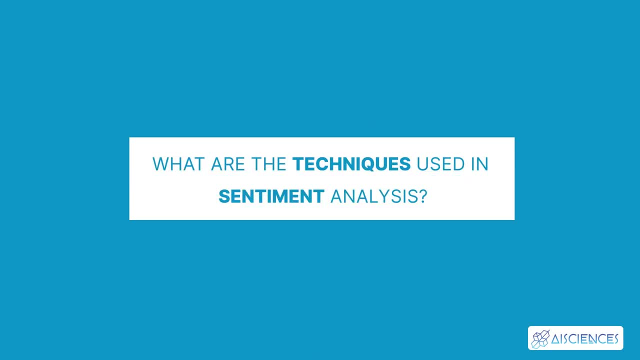 Now the question is: what are the techniques used in sentiment analysis? The first technique is rules-based sentiment analysis. It uses a dictionary of words labeled by sentiment to determine the sentiment of a sentence. Sentiment scores typically need to be combined with additional rules to mitigate sentences containing negations, sarcasm. 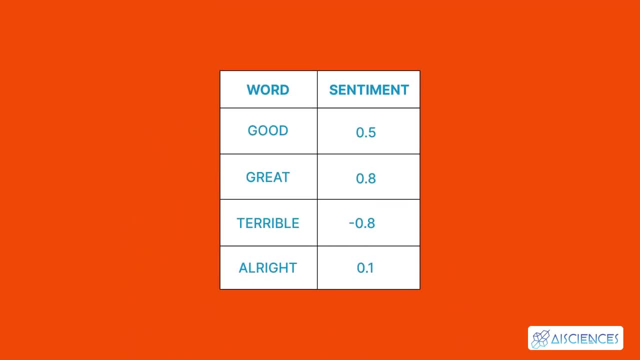 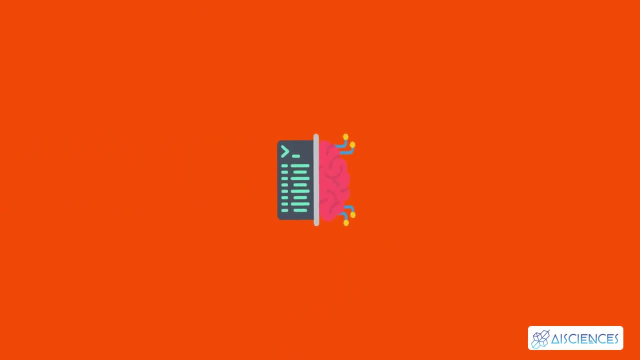 or dependent clauses. This is a sentiment dictionary example. Second one is machine learning based sentiment analysis. Here we train an ML model to recognize the sentiment based on the words and their order, using a sentiment label training set. This approach depends largely on the type of algorithm. 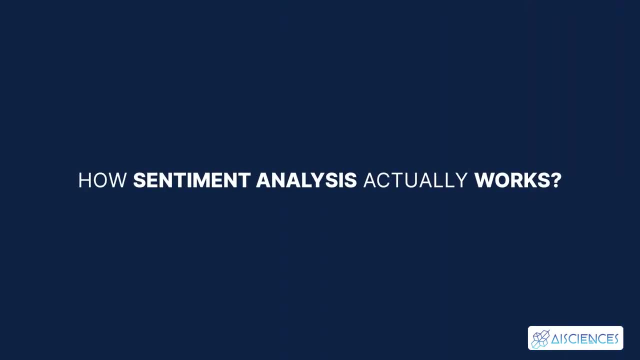 and the quality of the training data used, How sentiment analysis actually works? The answer to this question is: traditional sentiment analysis involves using reference dictionaries of how positive certain words are and then calculating the average of these sentences. For instance, you could use a dictionary to enhance the品's. 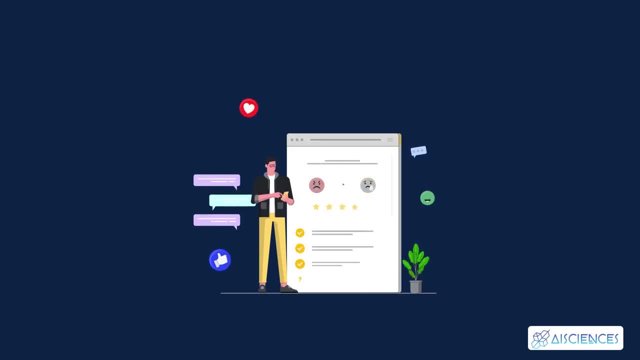 resolution to a certain level by calculating the number of sentences in terms of content. The English word for sentiment analysis is sentiment, a very common term forけど, frequently used to describe the price of a product. It can be used to draw from hearts. 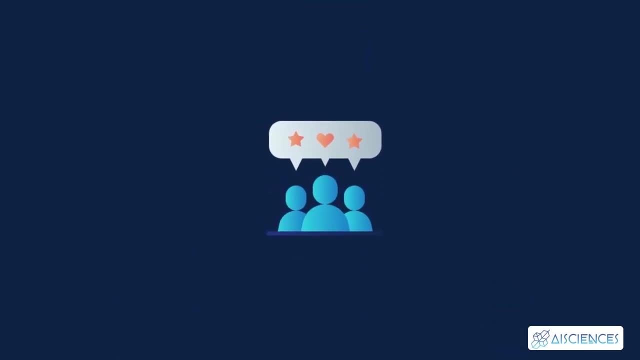 or to시 or touation, or to eat, or to go to the store or to sell to sell. The reason for sentiment analysis is that text can be used to analyze the purpose of a product, or to notice what it's doing, or to assess how we see it. Can sentiment analysis be used to generalize? sentiment analysis: No. Thank you for watching. I hope this video was helpful. Please like and subscribe to our channel. Don't forget to share this video with your friends and family. Thank you for watching. See you in the next video. Bye. 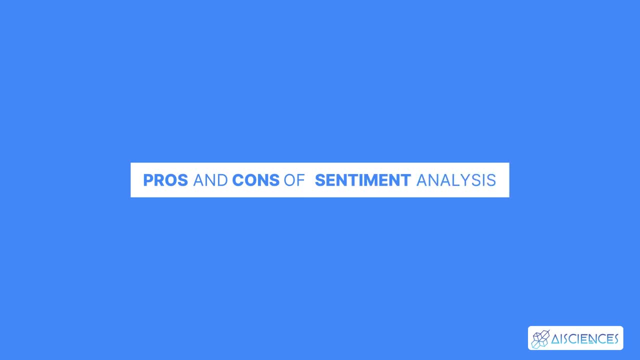 but do you know what are the pros and cons of sentiment analysis? By using sentiment analysis, you gauge how customers feel about different areas of your business without having to read thousands of customer comments at once. If you have thousands of feedback per month, it is impossible for one person to read all of these responses. By using sentiment analysis, 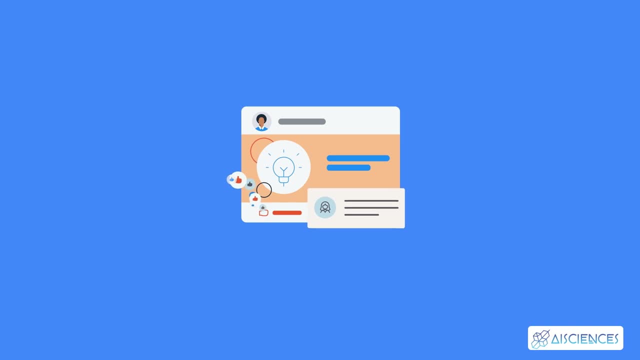 and automating this process, you can easily drill down into different customer segments of your business and get a better understanding of sentiment in these segments. Where sentiment analysis can help you further is by identifying which of these comments you should read If you're interested in learning more about starting a machine learning and AI career.